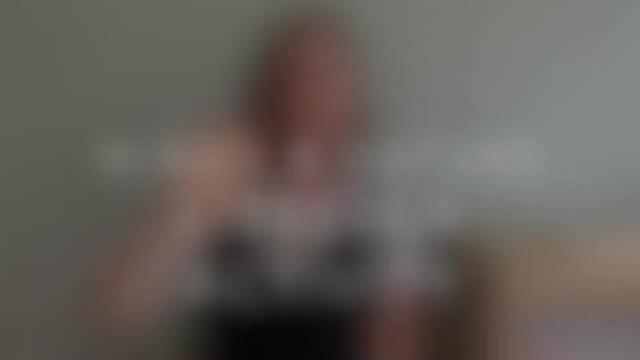 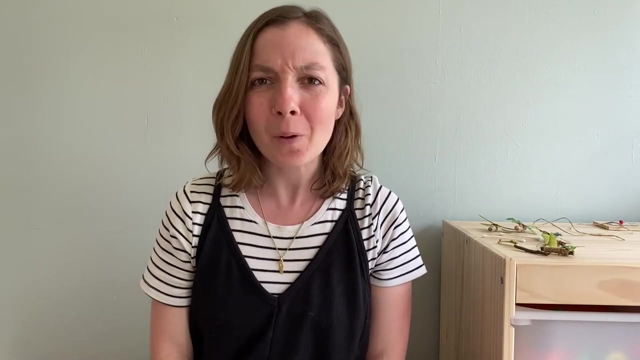 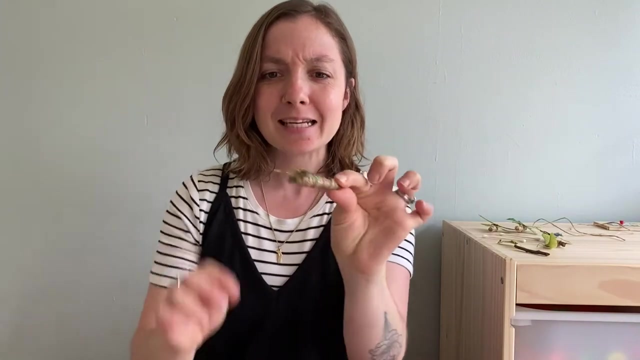 Hola amigos, I'm so excited to show you about the libelulas that I made the other day. Libelula- What could a libelula be? Hmm, Does this remind you of a type of insect? Tiene, cuatro alas Alas. are the wings right that help it fly? How many is cuatro in? 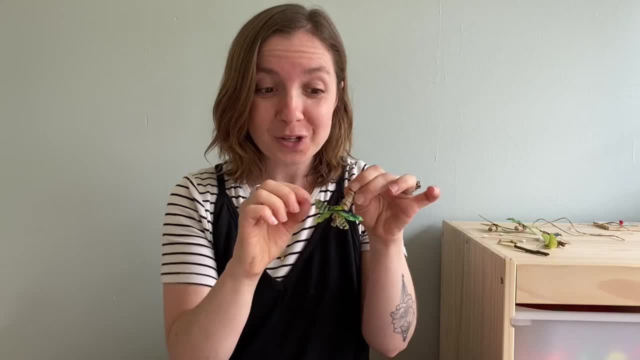 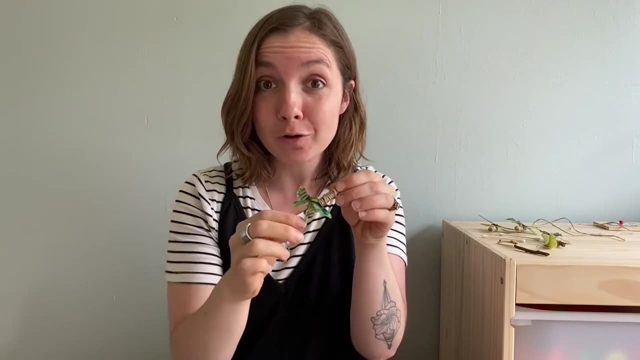 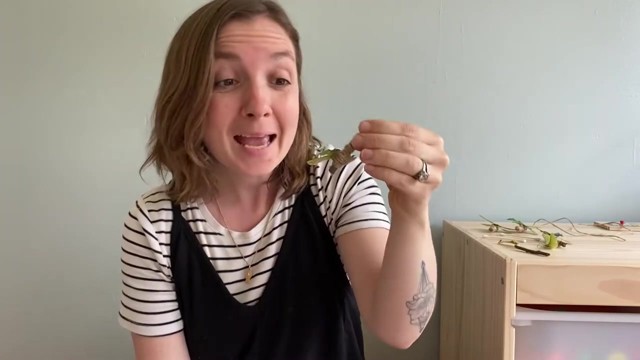 Español. Will you count with me Uno, dos, tres, cuatro, Cuatro. It has four wings and they're usually really colorful right? Tienen muchos colores. What colors does this one have? Yo veo azul, rojo y un poquito de verde, and a little bit of verde, a little blue, red and green. 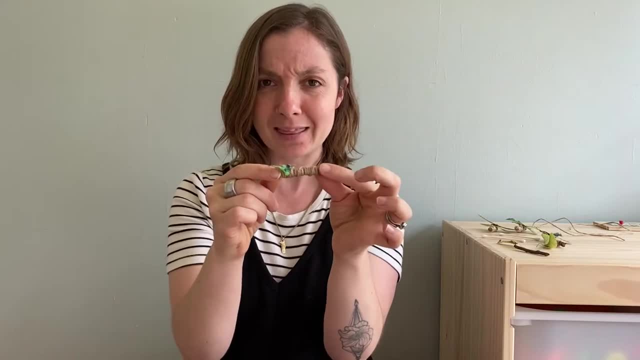 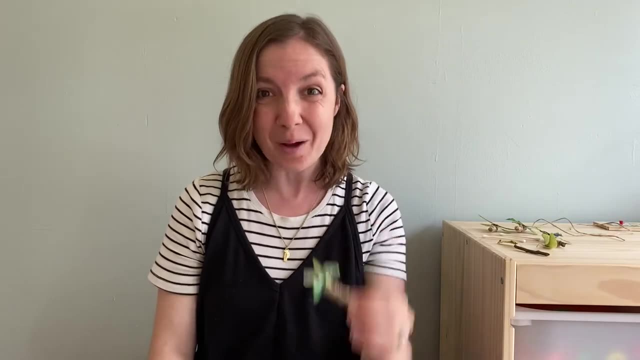 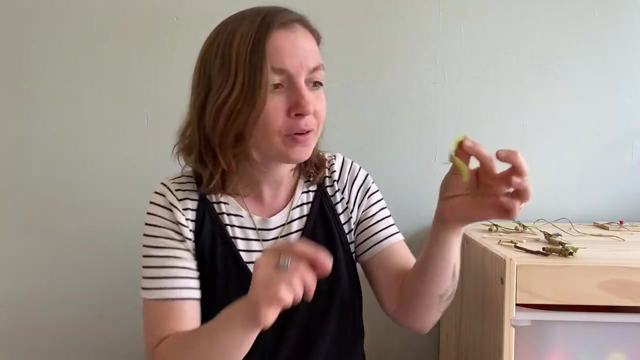 And it has un cuerpo muy delgado. It has a thin body. It's a dragonfly, Una libelula. Can you say libelula, Awesome Libelula. Can I show you how I made them? I was walking around outside and I found one of these. Have you seen these in your backyard? 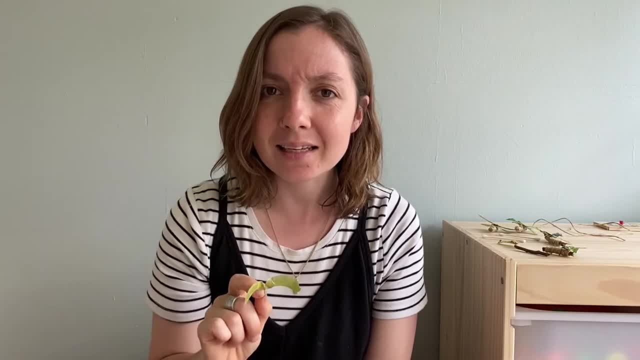 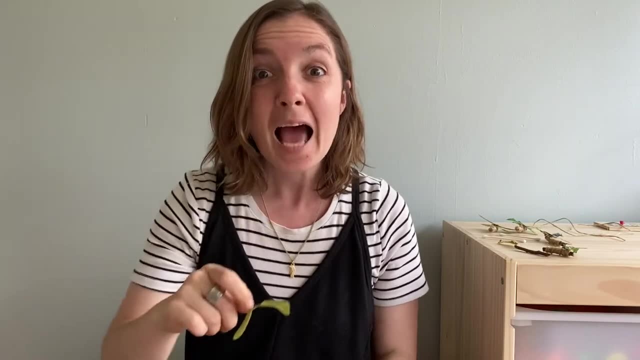 before Es una semilla, It's a seed. Is it a seed to una flor muy pequeña, to a little tiny flower? No, Es una semilla de un árbol grande, of a big tree. What kind of tree is it? Do you know? 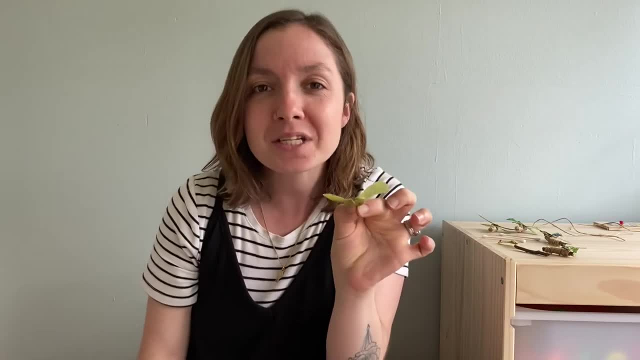 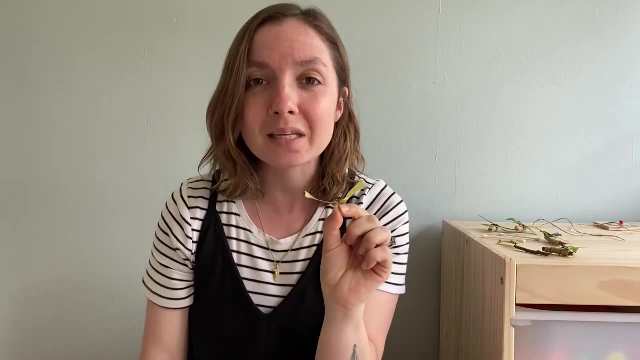 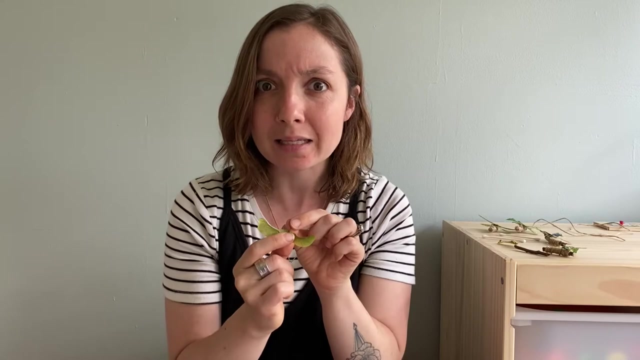 A maple tree. En Español se dice arce, Arce. So this is a semilla de arce, a seed of a maple tree, Semilla de arce. And I was thinking, wow, these would make some beautiful wings if I could make. 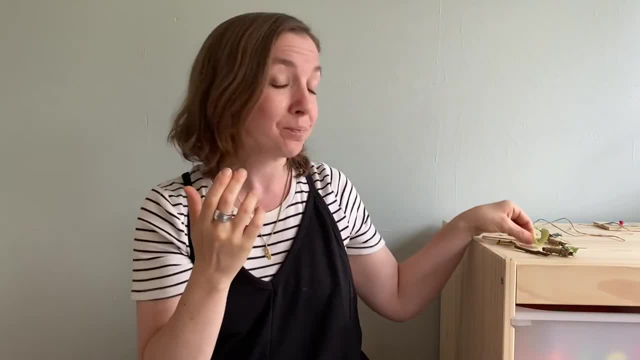 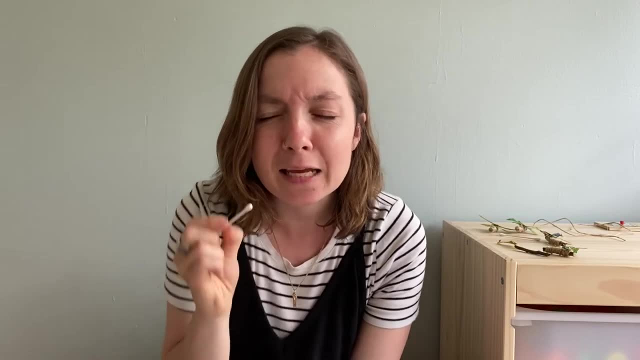 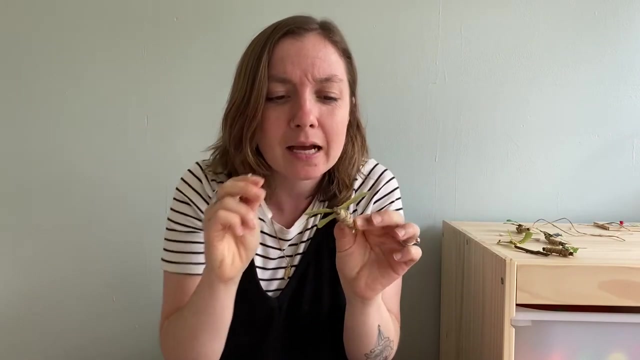 a dragonfly with them. So what I did is: I got my semilla- Do you know what this is? I got a q-tip for painting Very, very delicately, And I took my q-tip and I painted just these little tiny dots. I was. 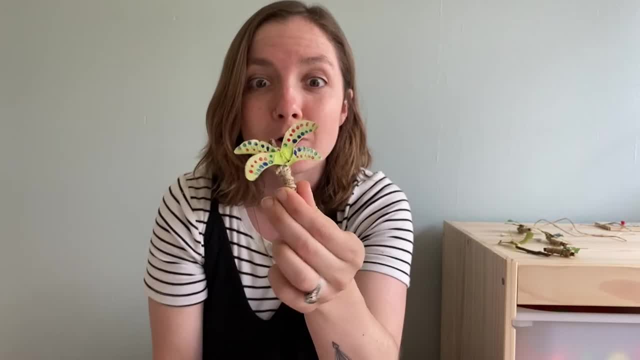 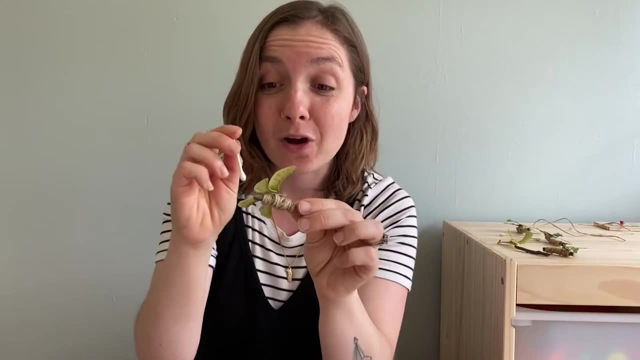 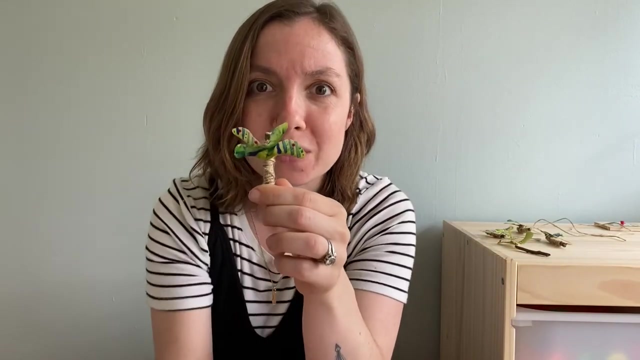 trying to be very, very careful and mindful of what I was painting, And so I wanted to use my q-tip to do tiny dots, some lunares- right, Those are called dots lunares. Or sometimes I wanted to make rayas, these stripes, Or my kids. they loved just making this cool tie-dye pattern. 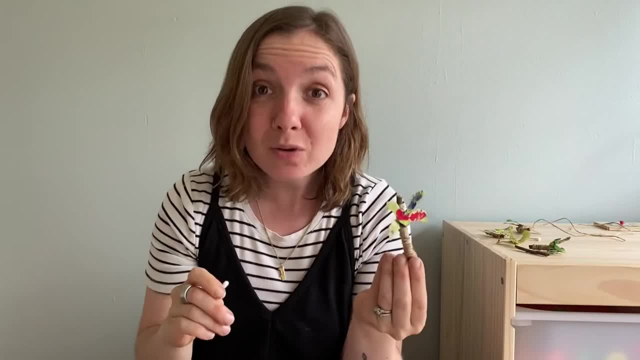 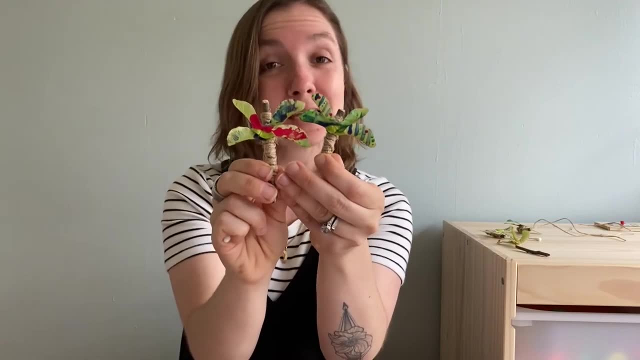 with it right, And mixing all the colores, But we used the same colores. Can you notice which ones we used? Azul, rojo y verde, Blue, red and green, But you can use any colors that. 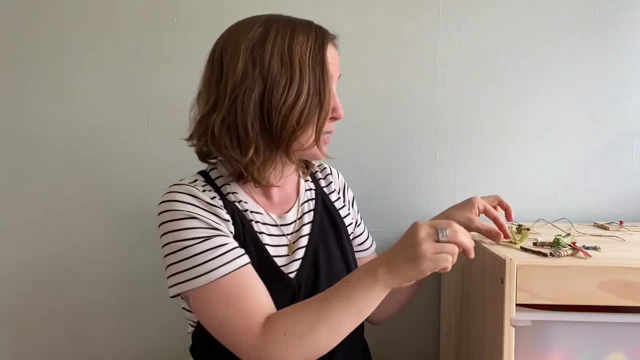 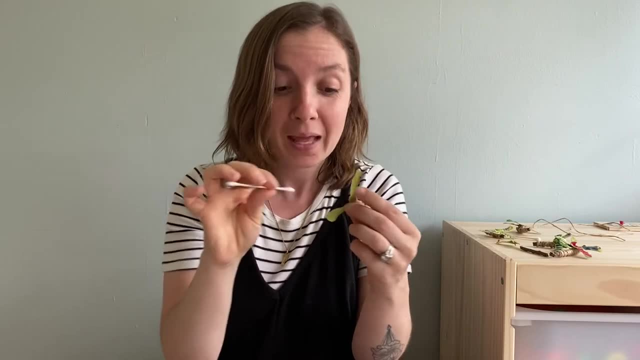 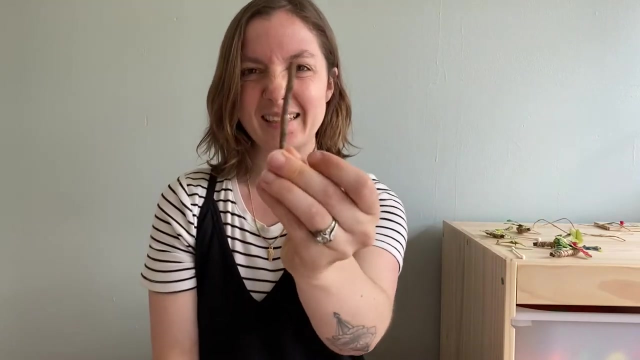 you want. So first we painted our semillas, right, Pintamos. That means that we painted, Pintamos las semillas. We painted them And then we let them dry And then, when they were all dry, we took a palo- What is this in English? Un palo, A stick. We took a little palo and I took some. 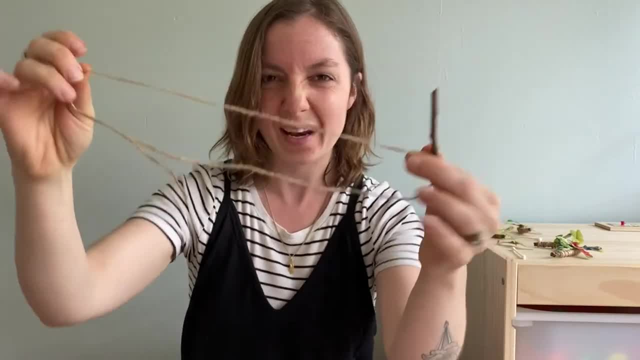 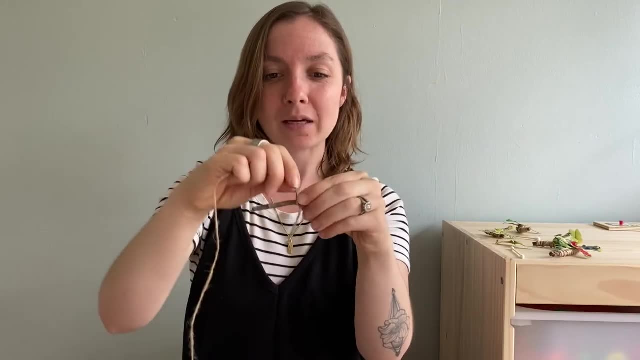 cordero. Do you know what cordero is? This is twine. Have you seen it at your house? maybe in the garden or for other art projects? I took the cordero and I wrapped it all around the palo. 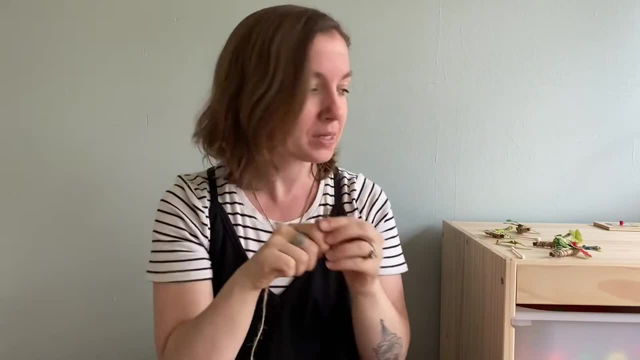 I wrapped it all around like this, And when it was done, I took my painted alas. and I wrapped it all around the palo. And when it was done, I took my painted alas, and I wrapped it all around like this. And when it was done, I took my painted alas. 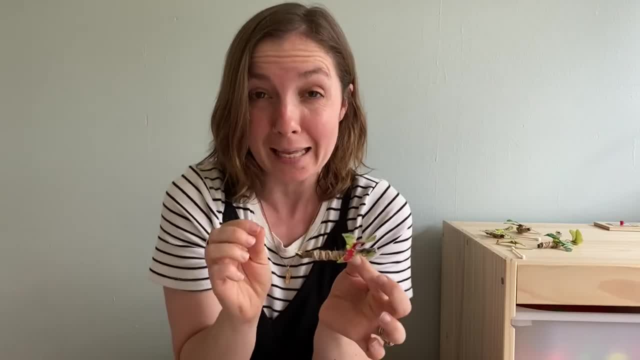 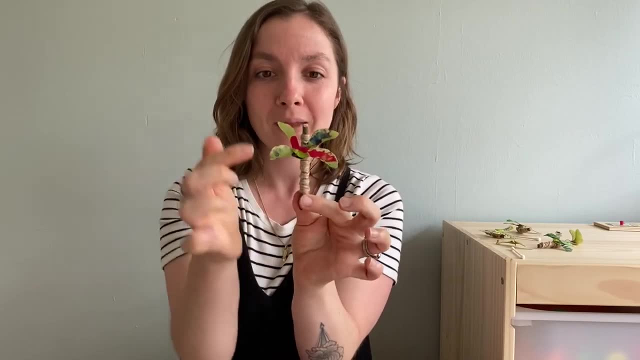 and I used a special glue that gets really, really, really caliente, So hot, So hot. And I used it's called hot glue- and I glued the libelula wings on and I crisscrossed them like that to make sure that they had four. alas, right Una libelula. 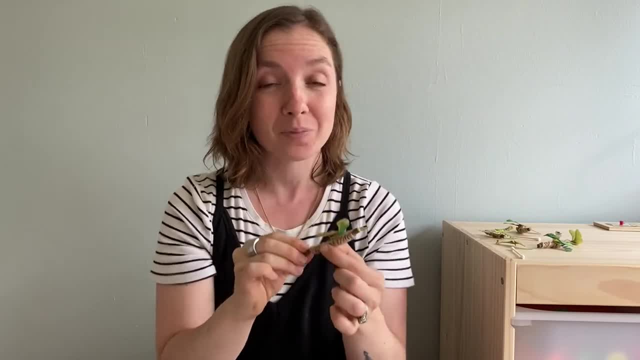 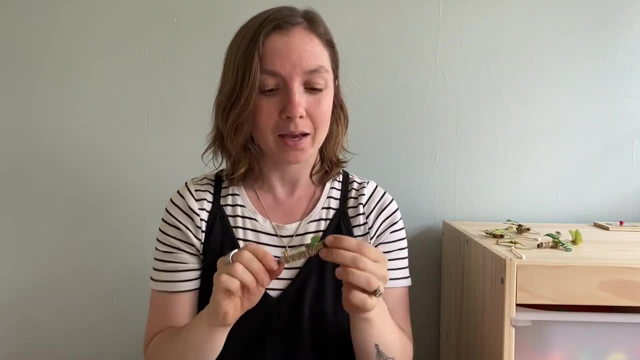 Are you gonna make some this week? I would love to see them. Can I review the words that we learned today? Libelula- Libelula is dragonfly, And then we talked about what helps the dragonfly bola. Libelula is dragonfly, And then we talked about what helps the dragonfly bola, What helps it fly. 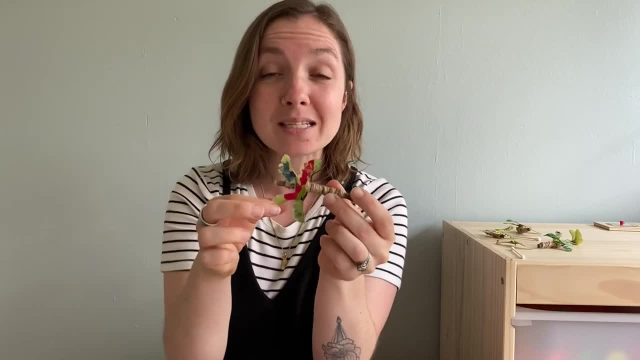 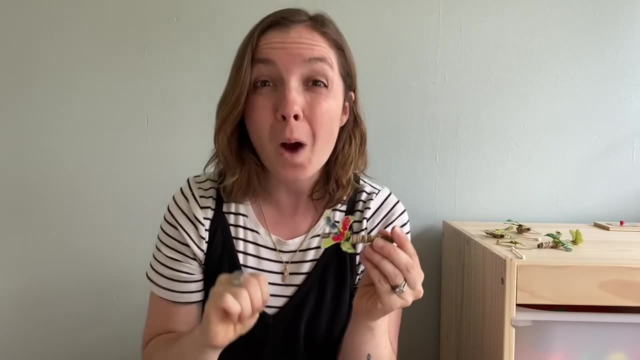 It has alas, Alas. These are its alas. Can you say alas, Awesome, It's alas. And how many alas does it have? Cuatro, In Espanol it's cuatro. Can we count them one more time? Uno dos tres.